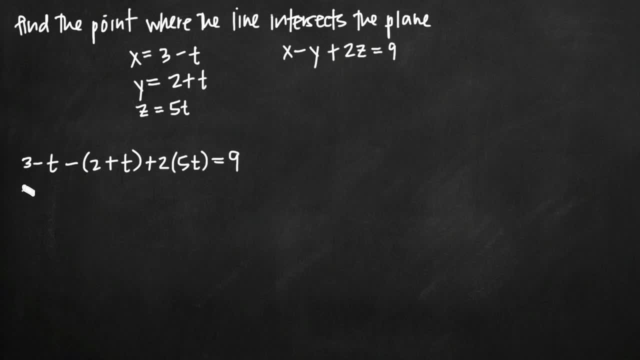 So we're going to get 3 minus t. When we distribute this negative sign, we'll get minus 2 minus t. 2 times 5t is 10t, so we'll get plus 10t is equal to 9.. Now we want to consolidate our t values and our constants. 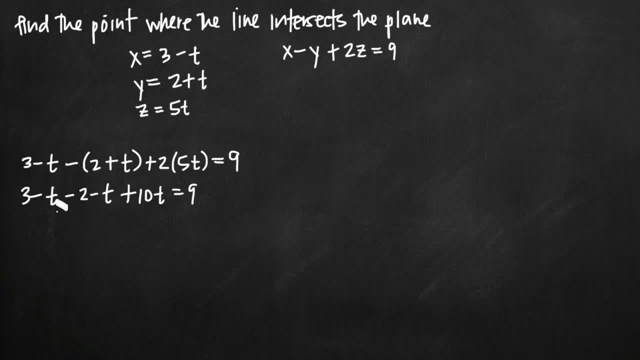 So here on the left hand side we have minus t, minus t plus 10t. That's going to give us 8.. Now we want to consolidate our t values- 8t- on the left hand side. We want to consolidate our constants on the right. 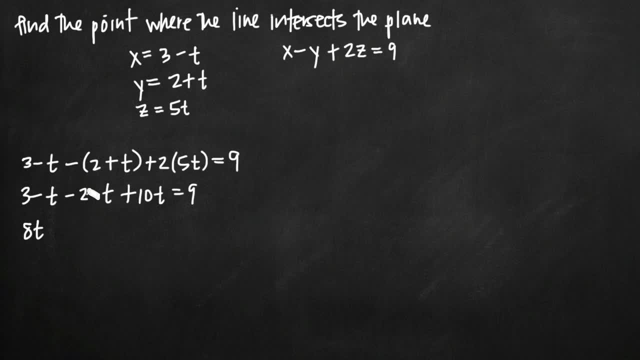 So we have 3 minus 2, which is equal to 1.. We want to go ahead and subtract 1 from both sides, which will cancel the constants on the left. We'll be left with a value of 8 on the right hand side. 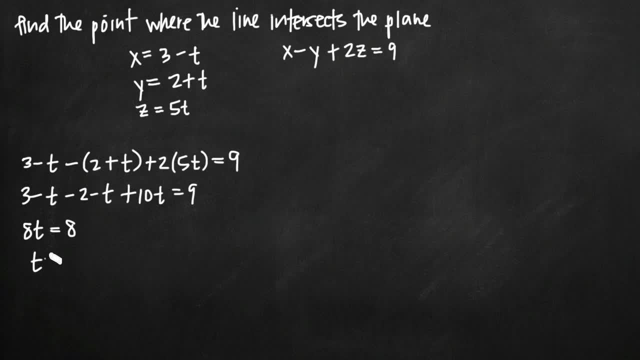 So 8t is equal to 8. dividing both sides by 8, we get t is equal to 1.. This is the value of the parameter where the intersection occurs between the line and the plane. Now, in order to find a coordinate point in terms of x, y and z where the intersection 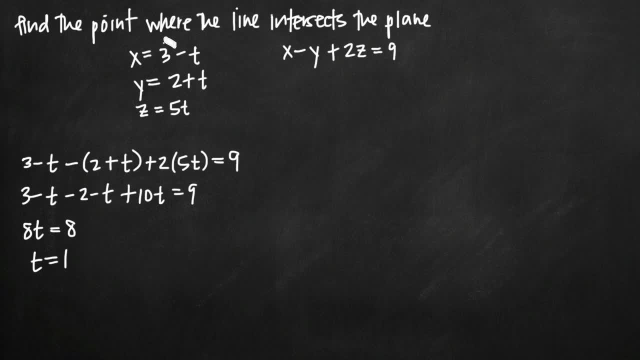 occurs. all we need to do is plug this parameter value into the parametric equations of the line. That will give us values of x, y and z that we can plug into our coordinate point. So here's what that looks like. Let's say we plug in 1 for t as the parameter value. 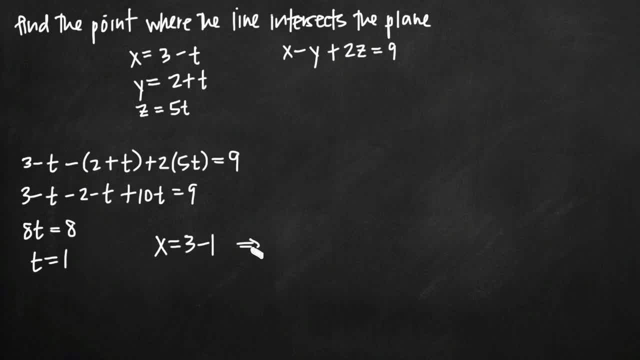 We'll get x is equal to 3 minus 1 or x is equal to 2. here We'll get y is equal to 2 plus 1 or y is equal to 3.. And we'll get z is equal to 5.. 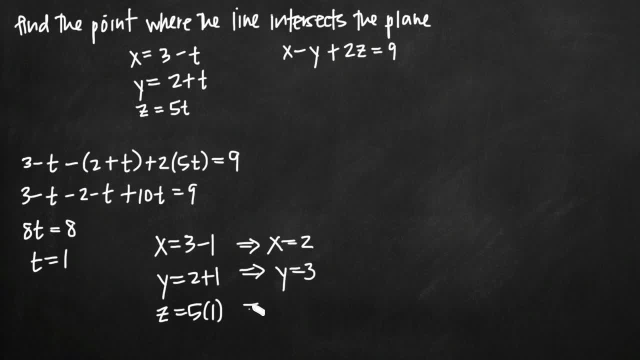 We'll get: z is equal to 5 times 1, or z is equal to 5.. So this becomes now our coordinate point 2,, 3,, 5, where the intersection occurs. All we need to do just to verify that we did everything correctly is plug this coordinate. 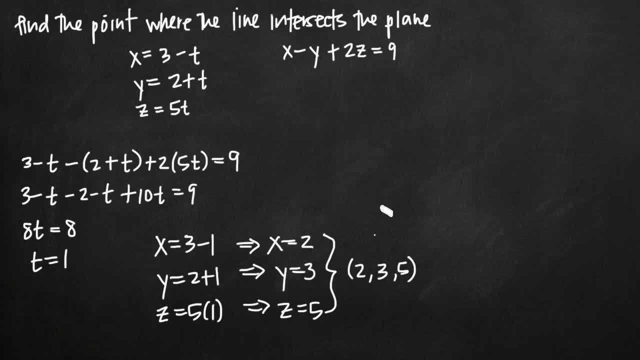 point into the equation of the plane. If this coordinate point satisfies this equation, then we know that we've done it correctly and we have a true point of intersection. So let's just go ahead and plug in 2., 3., 5..